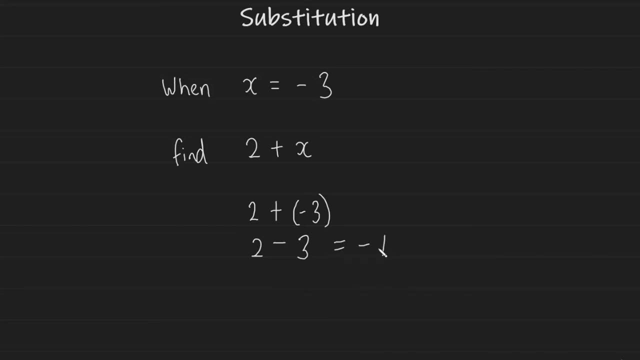 which is negative one, And that's the answer there. Okay, let's look at a slightly more complicated expression. So here we have two x squared minus ten, and we're going to do the same thing that we did in the last example: Wherever there's an x, I'm just going to replace the x with brackets minus three. Notice how I keep. 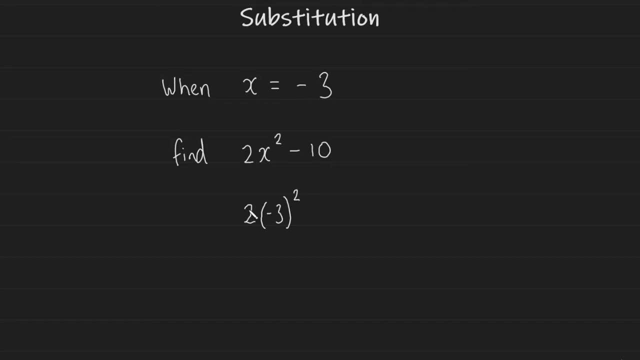 all of the operations outside of the x, outside of the brackets. They remain outside of the brackets and then we have the minus ten at the end. So now you're going to see why this is very powerful. Here we have minus three to the power of two, and then, multiplied by two, The operations follow. 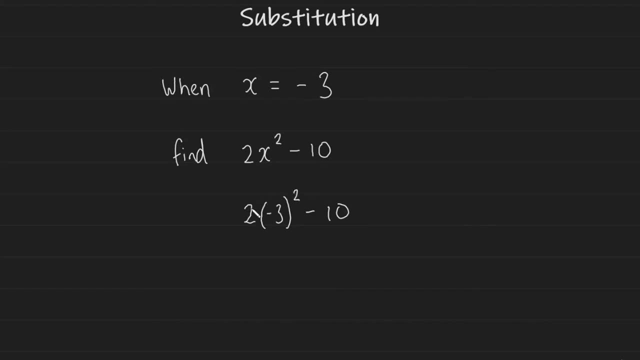 bid mass, So indices or powers before multiplication, because this two is being multiplied onto the minus three. So we're going to have minus three to the power of two, which is minus three times minus three, which gives us nine, and that gets multiplied by two, which gives us eighteen, and then we minus ten. 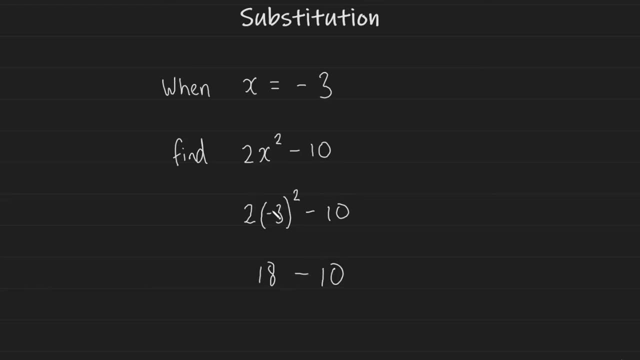 Now, if you want to take your time with the calculations, that's perfectly fine. If you are allowed to use a calculator, writing it exactly like this in your calculator will result in the correct answer. So if you don't have a calculator, you can highlight. 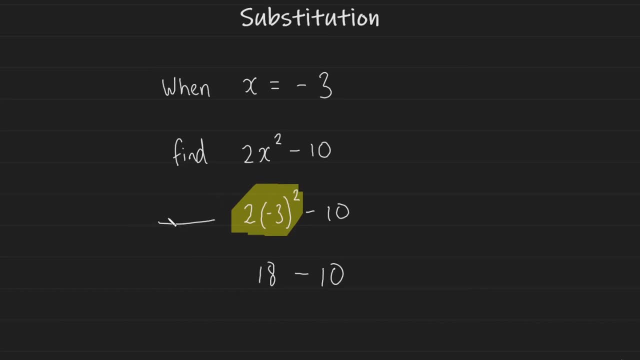 your work and take it to the side and do the calculations there. So I have minus three squared and then multiplied by two. So this is going to be nine because the power acts on it first and then it's being multiplied by two, which gives me eighteen. So you could do that if you wanted to. 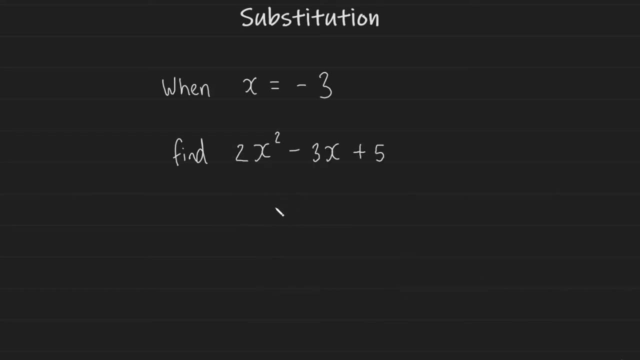 And the answer will be eight. Okay, now let's take a look at a slightly more complicated quadratic. So here we're going to have two brackets, three squared, So we're just replacing the x with a minus three, and then it's going to be minus three brackets, negative three plus five. And there it is. 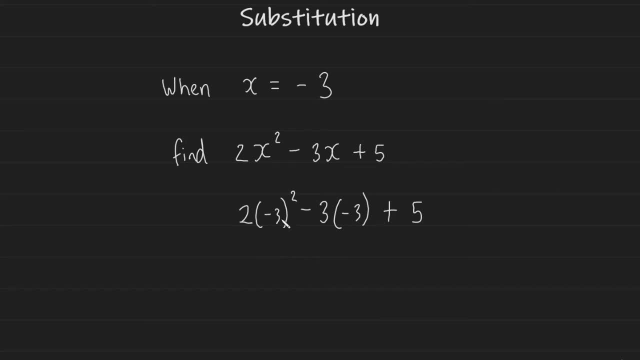 Inputting this into your calculator, as it looks, will give you the correct answer, Or you could just calculate it mentally: Minus three to the power of two, Minus three to the power of two is nine Times two is eighteen. Negative three multiplied by negative three gives us plus nine, And we have plus five at the end. 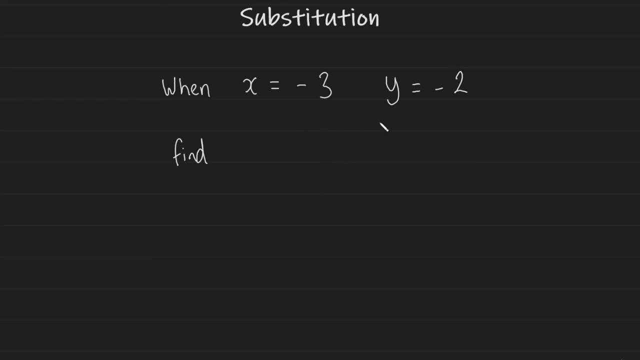 Adding all of this together will give us thirty-two. Now let's take a look at an example where you have two variables to input and see how we'll tackle this. We have two x y minus two x- y squared, So we're going to do two. Replace the x with the brackets minus three. Replace the y with the brackets minus two.